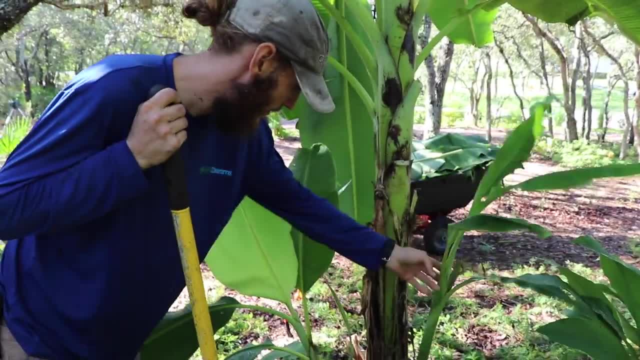 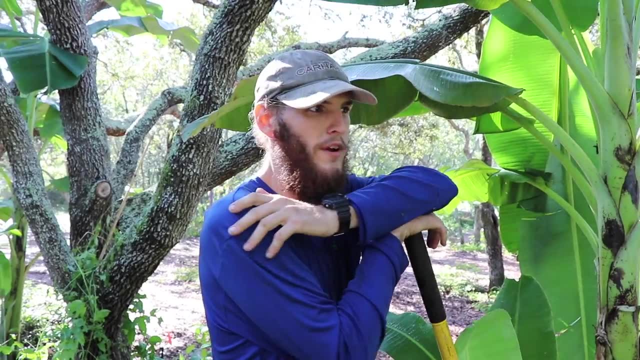 remove this one, but this is a good sword sucker here to remove for planting in other parts of the yard. cool, what would happen if we planted a water sucker? it just won't really grow too much. they uh kind of just won't ever fruit. it's real slow-growing. okay, well, that's not a regular shovel you got. 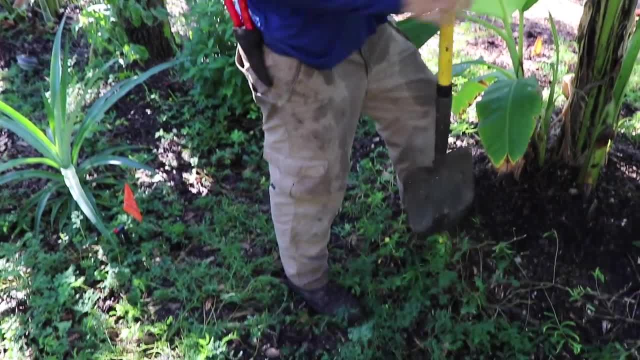 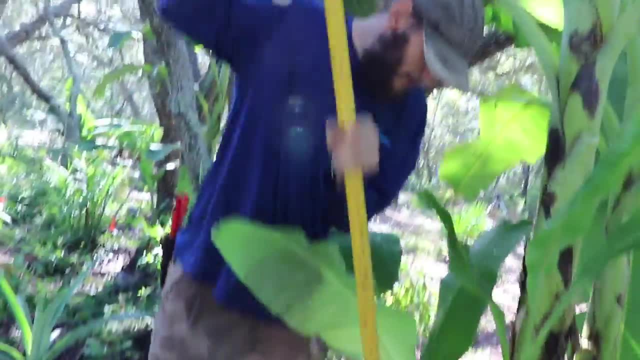 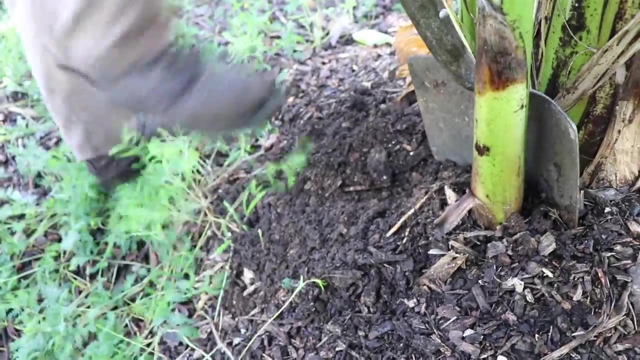 there either. huh, heavy duty pony shovel- that thing looks serious tools for the job. huh, oh yeah, all right, ian's a serious fruit forest, so this way you just want to slowly cut through here. I like to put shovel in there and kind of kick it with my boot here, and then basically what we're doing. 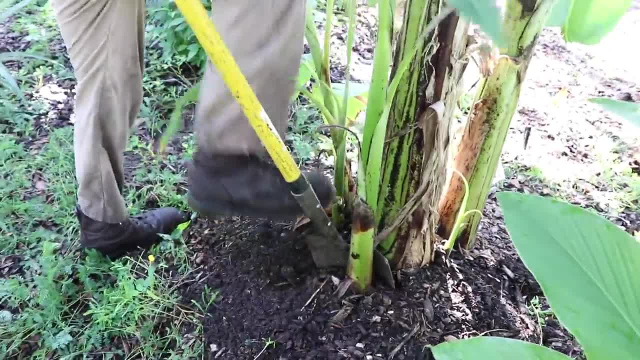 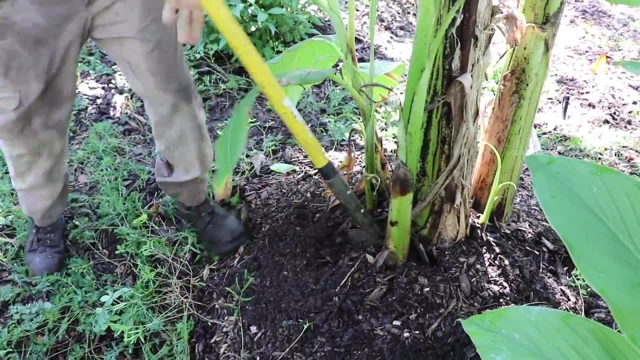 here, guys, we're taking one of the bananas off this and we're gonna go plant it. So you know, once you plant that first banana, all these little babies start to come up, you know. So it gives you other plants that you can separate and create more in the landscape. 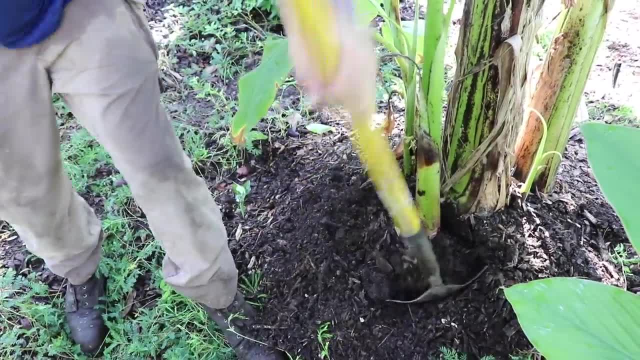 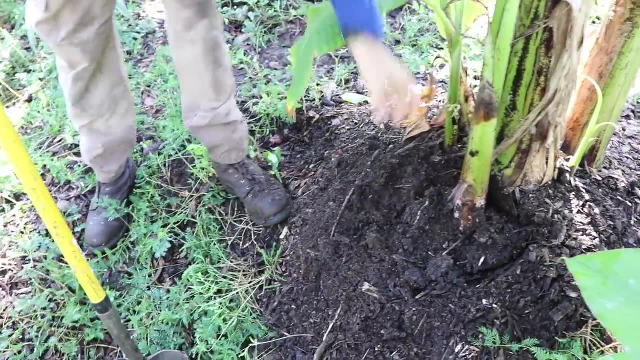 You can see Ian's just connecting that, you know sword sucker, or disconnecting that sword sucker from the corm. you know the heart of the tree. There we go. Wow, that is some soft soil. huh, That's some really good dirt here. 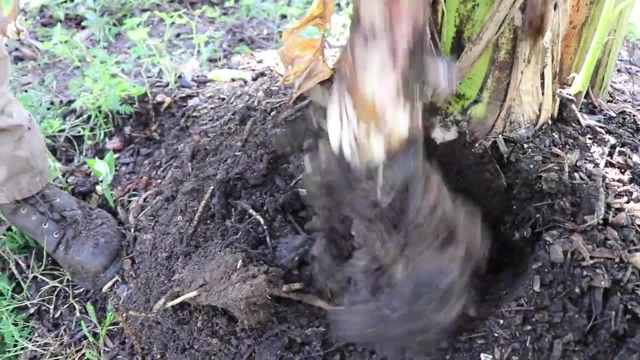 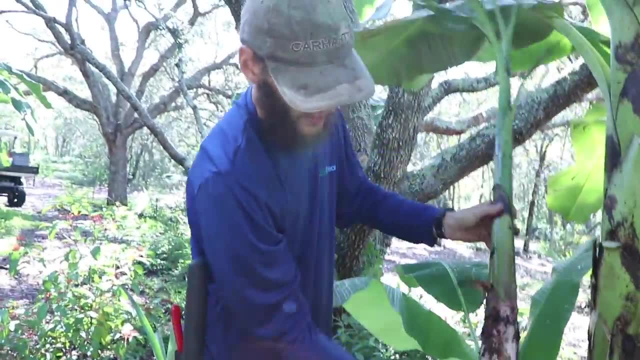 It's pretty rich here. This is not typical soil for Pasco County Whoa. So there you go. Basically, you just slice it off from the mother corm as roots. So what if you wanted to propagate that? What if you wanted to put that in the nursery? 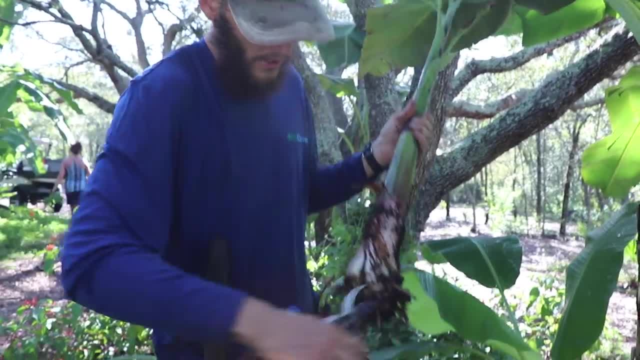 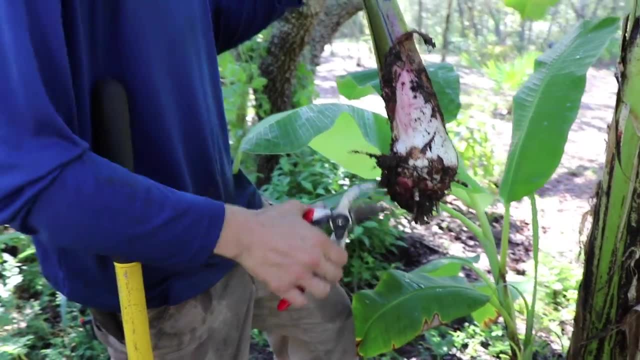 Any suggestions? We usually prune off the roots a little bit, kind of pop them off here. You let it dry out for a day or two, or straight into the soil. Yeah, let it dry out a little bit. Let it dry out a little bit. 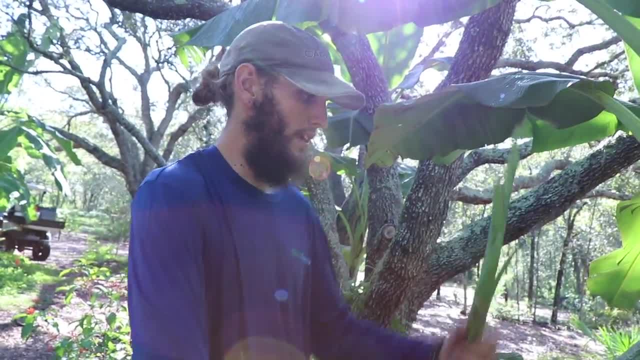 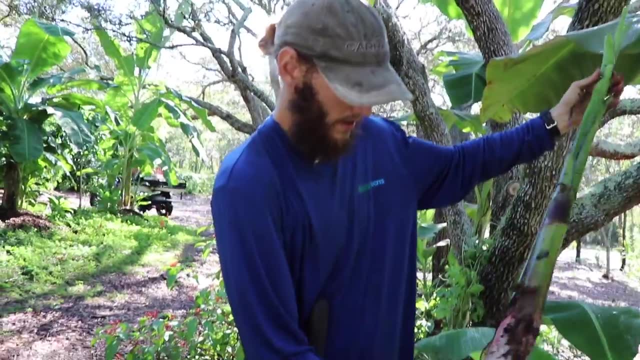 Also cut the leaves off the top here Helps it from getting too bad Drying out. okay, So look at that. We got another free banana. Free banana plant- huh, All right, free bananas- Zone 9B, Raja Puri. 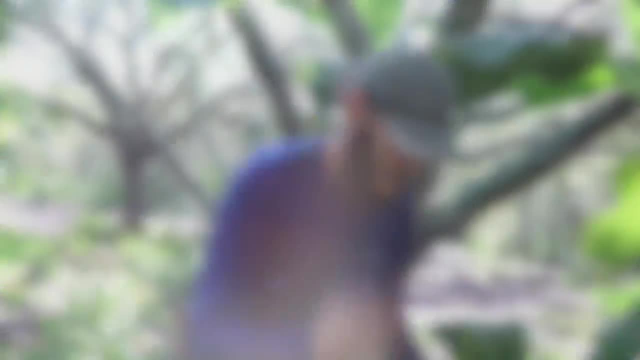 Wow, that is some rich soil. All right, Ian say: peace out, Peace out guys. If you guys enjoyed that video, please like, share, subscribe. Remember sharing is caring.